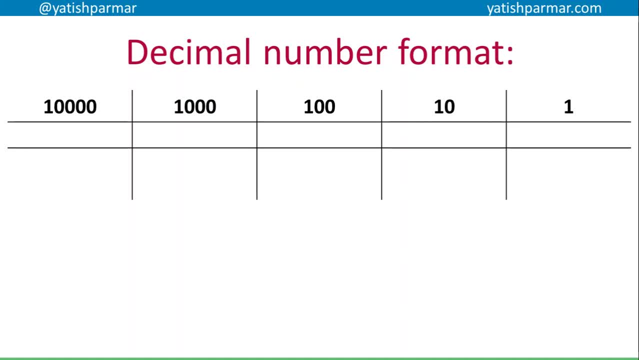 So the column placeholders are calculated using tens. So the right-hand column is 10 to the power of 0.. The next column is 10 to the power of 1.. The next column is 10 to the 2s, 10 to the 3s, 10 to the 4s, etc. 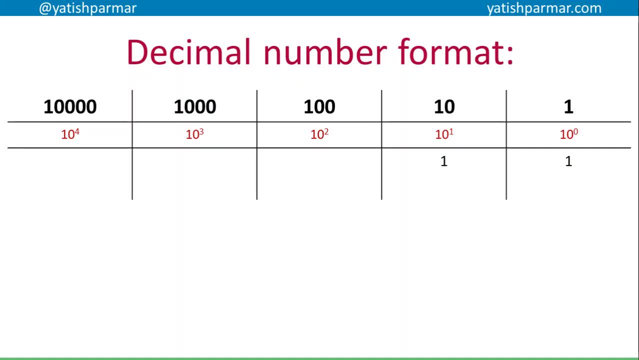 So when I'm storing a number, okay, putting one digit in each column, all right. and then that digit has a value based upon the column placeholder, All right. So 11 is going to be 110 and 111.. 108 is 101, no 0s and 8 1s, etc. 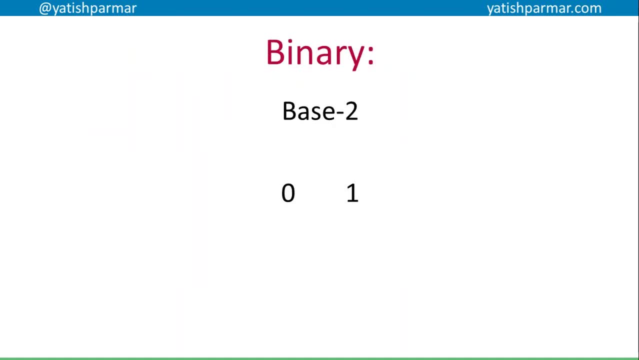 And we add up each of those individual values to get the total value for that number. Binary is a base 2 number system So, like in binary, we have 10 numbers, 0 to 9.. In binary we've only got two numbers: 0 and 1.. 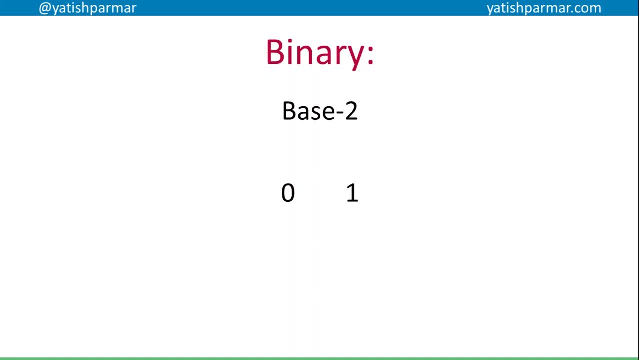 That's all the computer understands. We use binary because it corresponds to the two states that a transistor can be in, on or off, All right. So a binary number format will still allow us to store all the possible values, All numbers that we want to store. 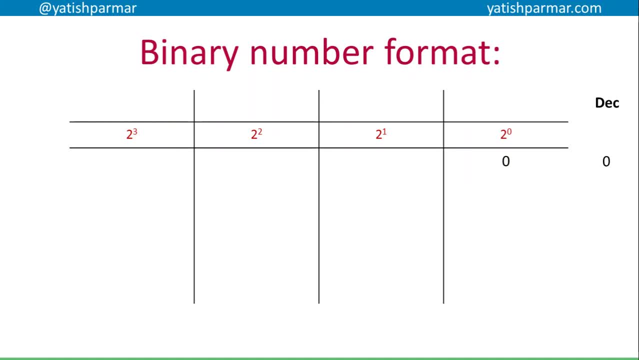 But the column placeholders are slightly different This time. instead of going up in 2s- sorry- instead of going up in 10s, we're going up in 2s, All right, So the decimal binary equivalent of each of those columns is going to be this: 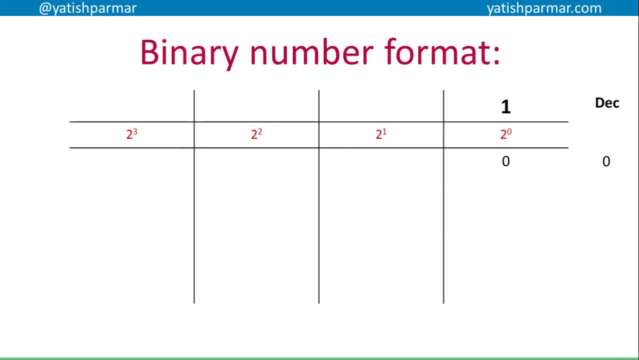 2 to 0 means I can store 0 or 1 in that column. The next column is 2 to the 1s. It's going to store 2s. The next column is 2 to the power of 2, so it can store 4s. 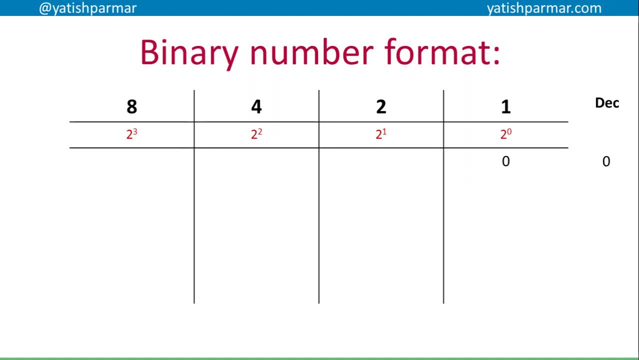 The next column is 2 to the power of 3, so it can store 8s. So how do I store all the possible values? Well, simply, if I want to store 0, it's just going to be 0,. okay, because I've got no 1s. 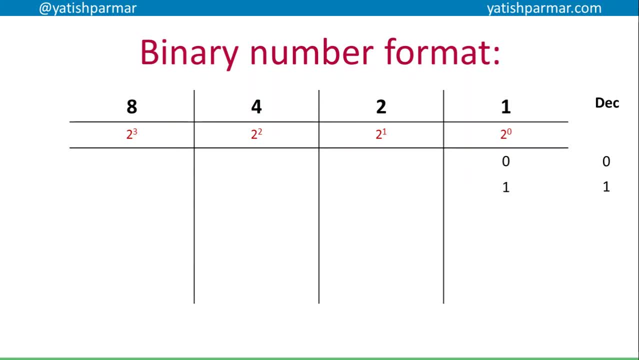 But if I want to store a 1,, then I'm going to put a 1 in that column, because one 1s is a 1.. What happens if I want to store 2? Well, I've got no 1s, but I've got one 2,. okay, because I've got a 1 in the 2s column. 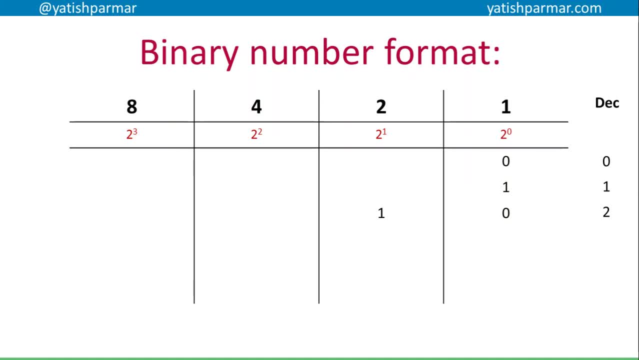 One times 2 is 2.. What happens if I want to store 3?? Well, I know I'm going to have one 2, but I've also got one 1.. And that gives me a 3.. If I want to store 9,, I'm going to have one 8,, no 4s, no 2s and a 1, because 8 plus 1 gives me 9.. 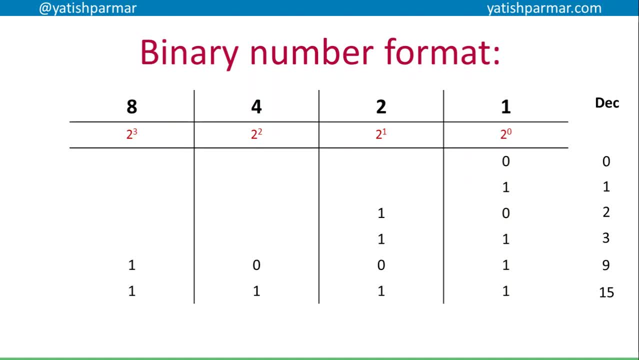 If I want to store 15, I've got an 8,, a 4,, a 2, and a 1, because if you add them all together you get 15.. Now we have names for the different size of number that we store in binary. 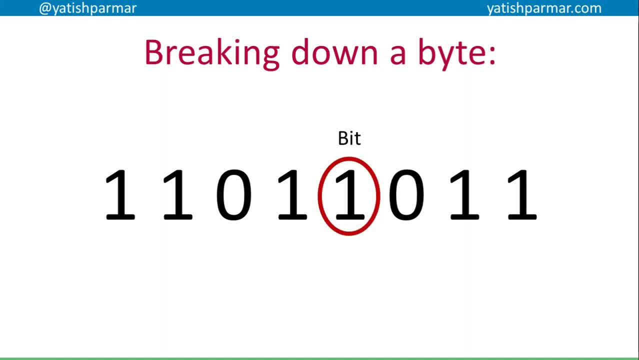 Okay, the smallest bit is literally a bit. Bit stands for binary digit. Okay, they compressed it together. all right, to make the word bit. The bit can only be. basically it's a single binary digit, so a 0 or a 1.. 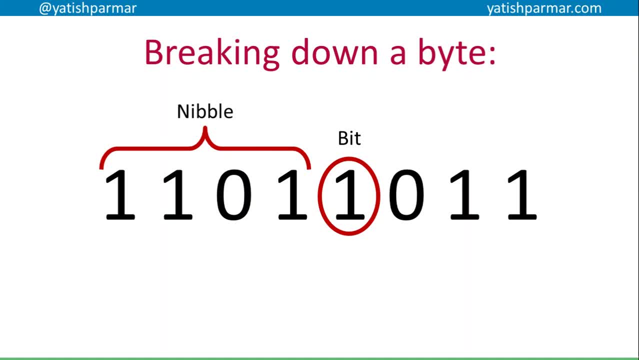 A nibble is 4 bits, And then the whole thing together, 8 bits make a byte, Okay, or 2 nibbles make a byte. whichever we want to do it. Nibbles are basically smaller than a byte. Now what you should be able to do. 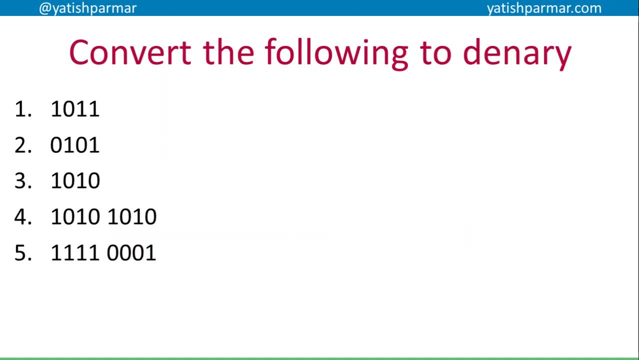 What you should be able to do, based on what we've just done, is convert the following binary numbers to denary: all right, If I were you, I'd hit pause, I'd have a go at doing the conversions and then hit play again and check the answers. 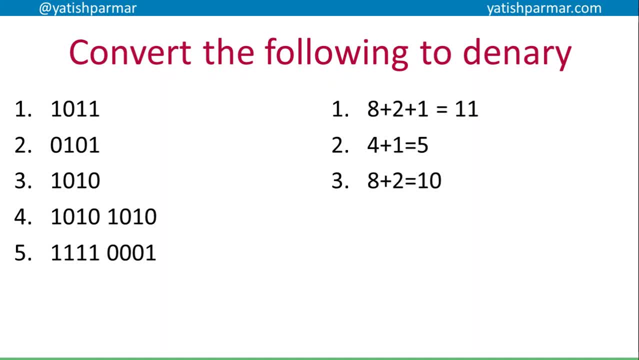 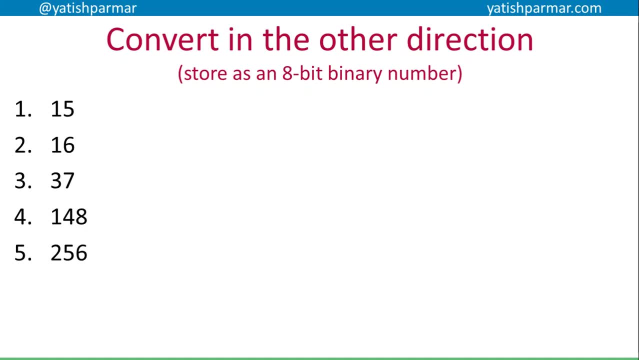 And assume when you came back, here are the answers for each of those different conversions. Did you get them all right? And I used to be able to flip in the opposite direction and store each of these numbers as an 8-bit binary number. 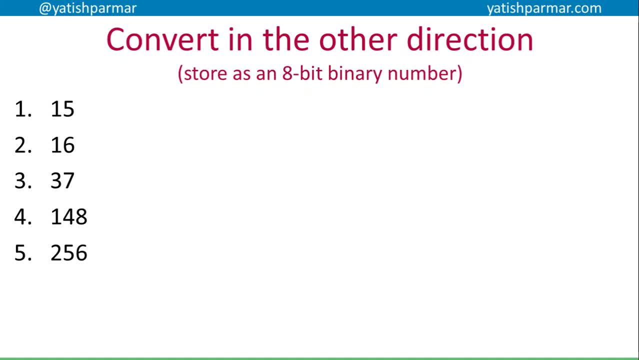 Okay, so hit pause And if you come back you should have figured it out that 15 is that this is 16,, 37,, 148, and now 256 cannot be stored in an 8-bit binary number. You need 9 bits to store it, okay. 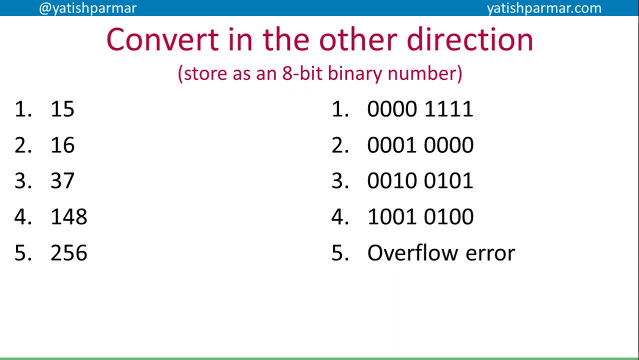 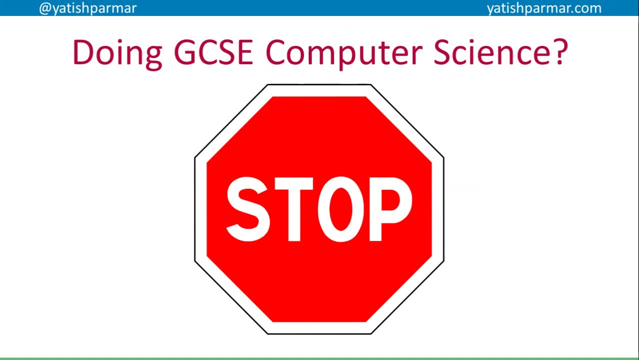 And therefore we get what we call an overflow error, because the number is now too large to be stored in the available number of bits. Now, if you're doing GCSE computer science, there's a bit where you stop. okay, You can go on to the next video about doing binary addition. 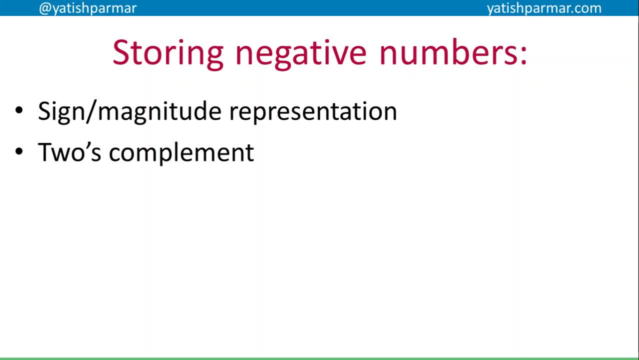 If you're doing ALF, we've got continue, all right. Now, if you want to store negative numbers, we've got two different ways of storing it. We can basically use sine and magnitude or we can use two's complement- all right. 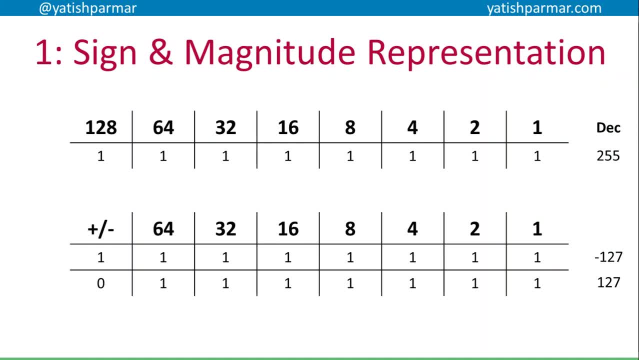 Sine and magnitude representation. basically, okay, is storing the sine in the number. I appear to have deleted a bunch of animations from this slide for some reason. Anyway, You have the most significant bit, which is the bit on the left-hand side. is actually storing the sine, okay? 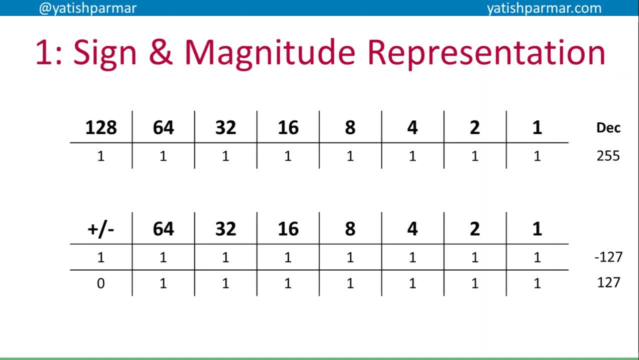 And then the rest of the number represents the magnitude of the number. The rest of the byte- sorry- represents the magnitude of the number. So if I want to store minus 127, I'm going to have 64,, 32,, 16,, 8,, 4, 2, 1, all added together gives me 127. 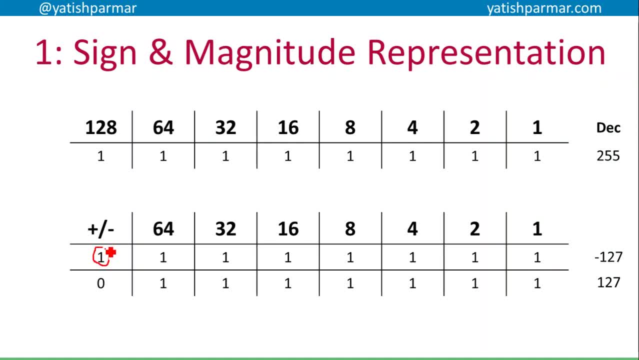 But the sine at the beginning of the number indicates that this is a negative number. Similarly, if I want to store 127, I'll still have a 64 plus 32, plus 16, et cetera, et cetera, et cetera. 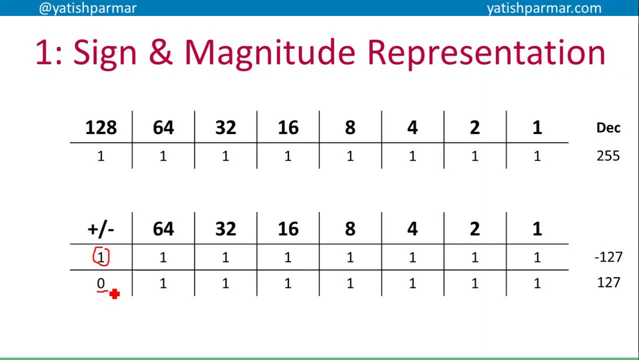 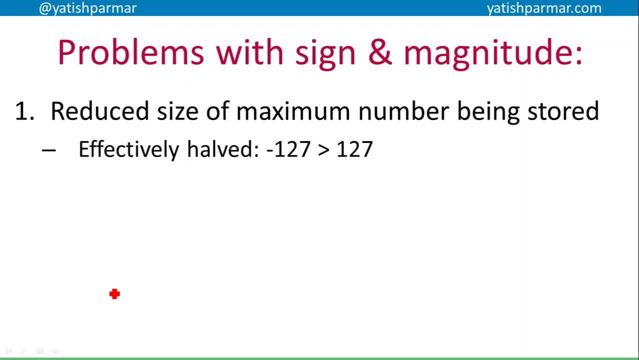 But this time the most significant bit is zero, indicating this is a positive number. Now there are some problems with sine and magnitude. okay, Firstly, we've just reduced the size of the maximum number that we can store. We've effectively halved it, so we can only basically store from minus 127 to plus 100.. 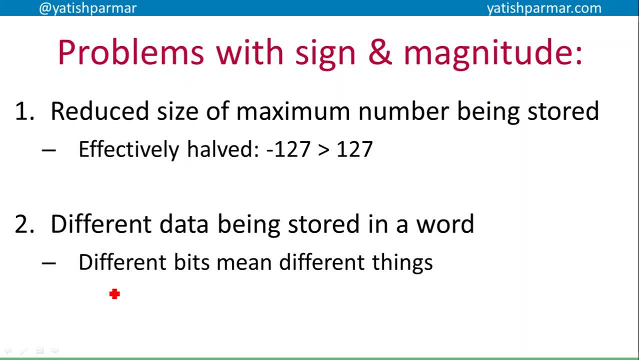 127,. all right. Also, there's different data being stored in a word, So therefore different bits mean different things. ie the most significant bit is represented in the sine and the remainder of the number represent a magnitude. This causes problems because programming logic then has to become more complicated in order to handle that. all right. 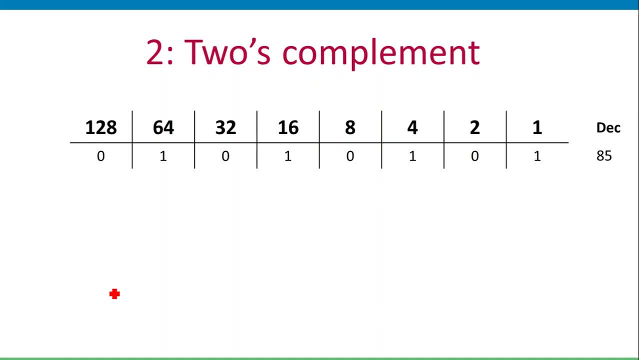 Second way of storing a negative number is to use two's complement. okay, So in the bottom table you can see this time actually, the most significant bit is still: is now a number, okay, But it's a negative number. 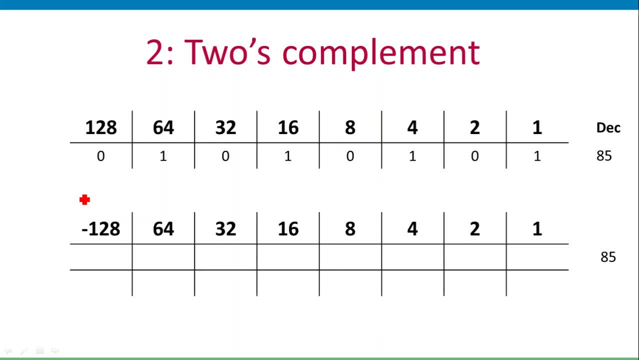 It's minus 128.. So that means that if I wanted to store, say, the value 85,, all right, I have no minus 128,, but I have a 64,. I have a 16,, 4, and a 1,, okay. 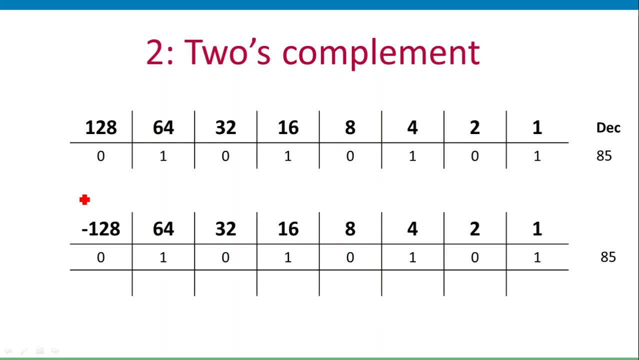 Because if you add 64 plus 16 plus 4 plus 1, you get 85. If I wanted to store minus 85, it'd be slightly different. I'd basically have a minus 128.. And then what positive.